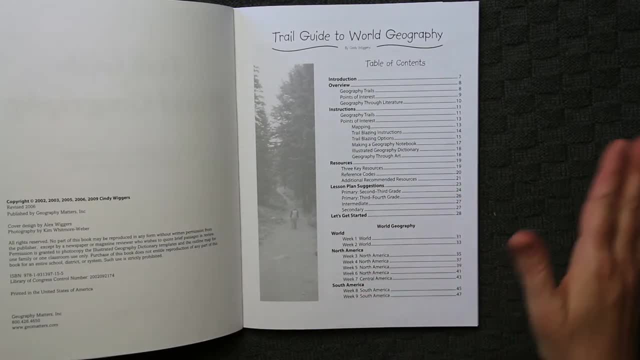 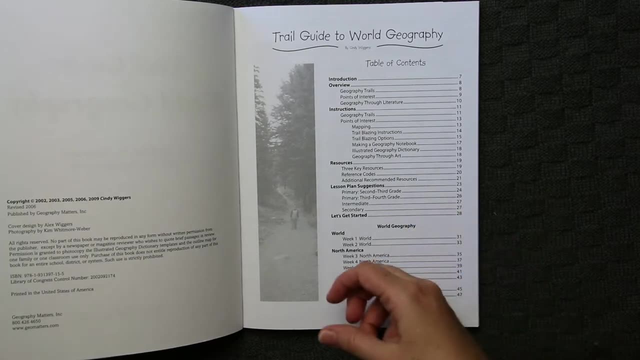 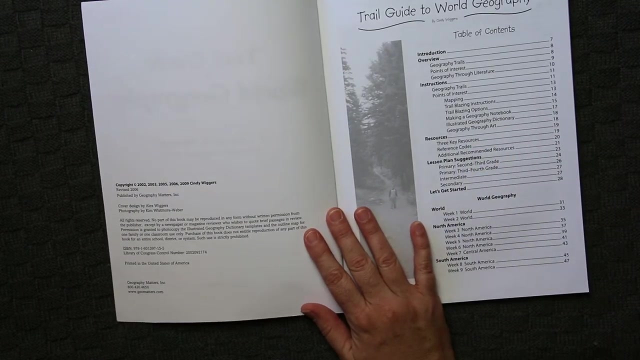 but to not be pigeonholed into having to teach lesson by lesson. The guide provides activities and assignments, along with map drills and atlas work. to spend 36 weeks of geography lessons, Okay, so let's jump in. So here, straight away, we have a detailed contents page clearly laying out where everything can be found. 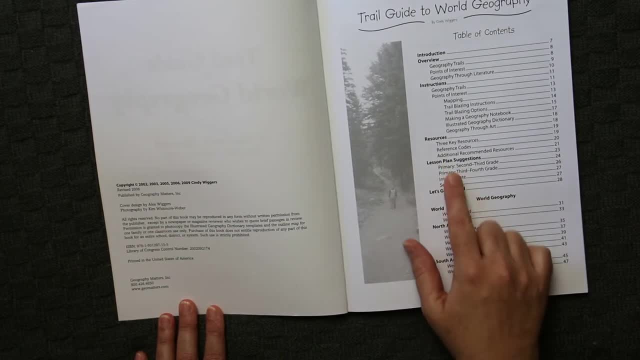 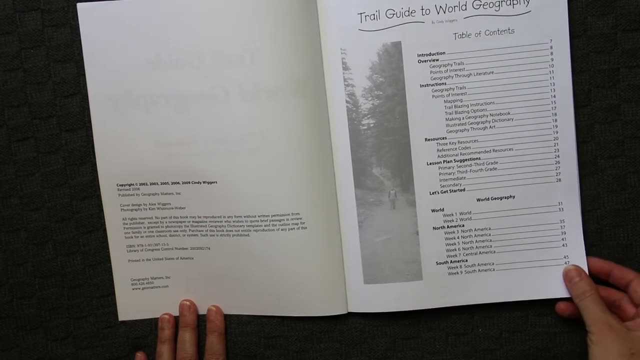 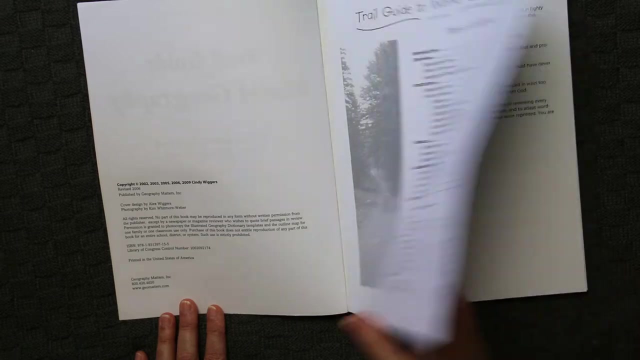 along with lesson plan suggestions for various grades, And then, of course, you get into the actual weekly activities and lesson blocks. So, as you can see here, you do spend most of your time in the Americas. Given this is an American produced program, I can see why There's also an option. 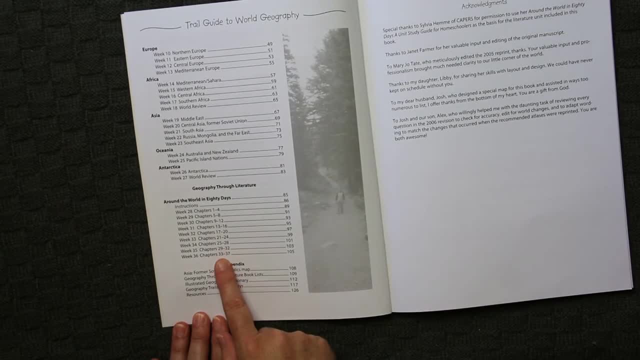 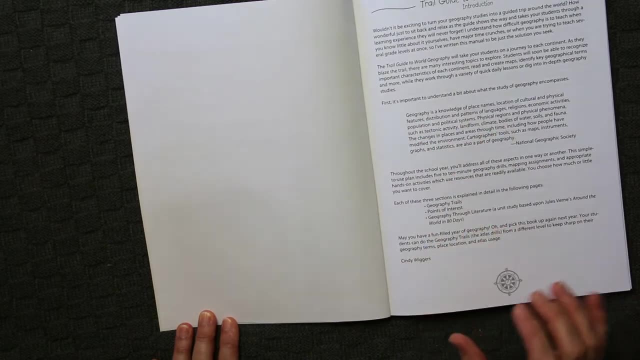 to work in the United States. So if you want to work in the United States, you can work in the United States. If you want to work in the United States, you can work in the United States. So that's a nice little addition there. The introduction explains the heart and mission of 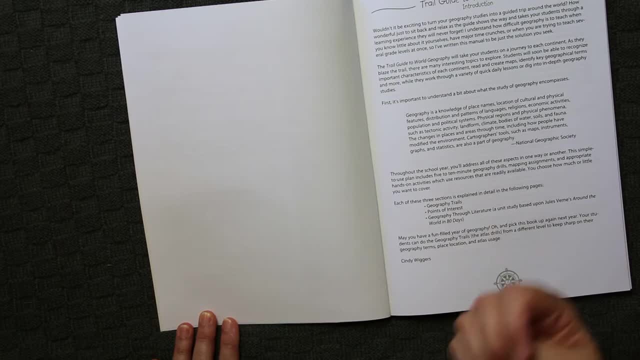 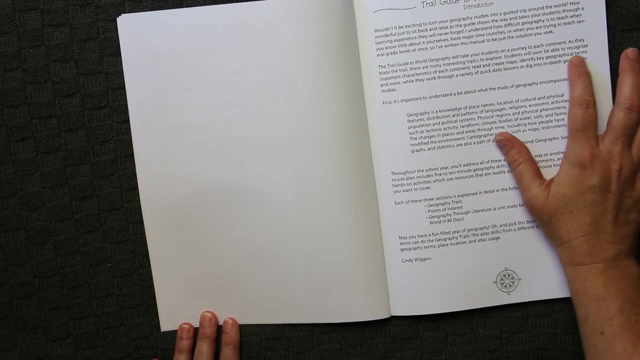 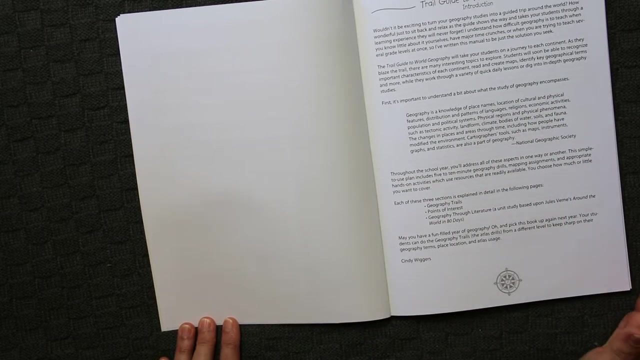 the guide and explains that your children will be taken on a journey to each continent. as they blaze the trail, There are many interesting topics to explore. Students will soon be able to recognise important characteristics of each continent, read and create maps, identify key geographical terms. 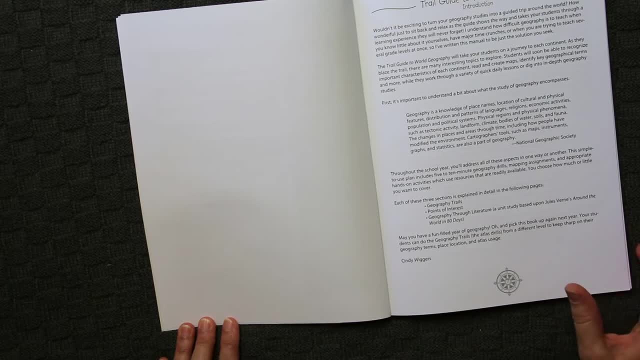 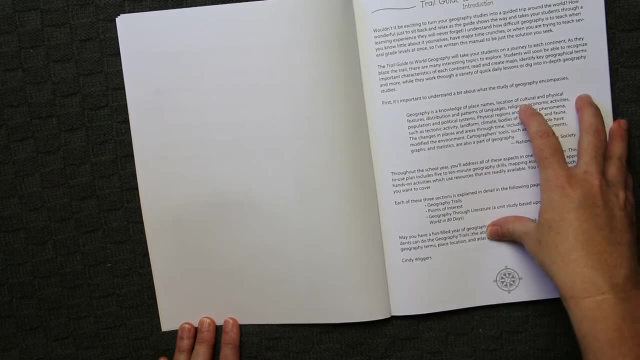 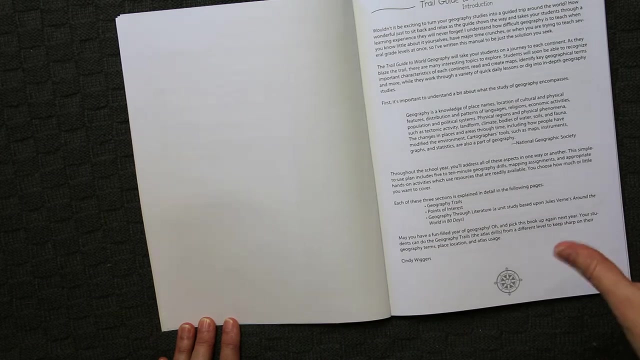 and more While they work through a variety of quick daily lessons or dig into in-depth geography studies, And that's something you'll see as we get further through. this is that this can actually be a really simple program that you use for literally five or ten minutes a day, or you can really flesh this out. 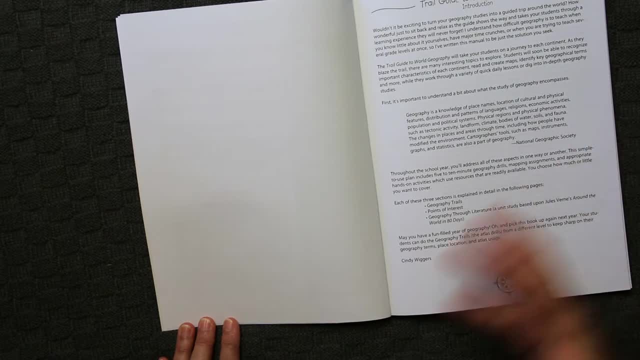 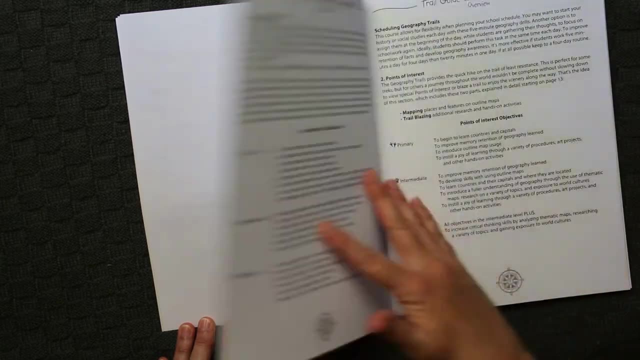 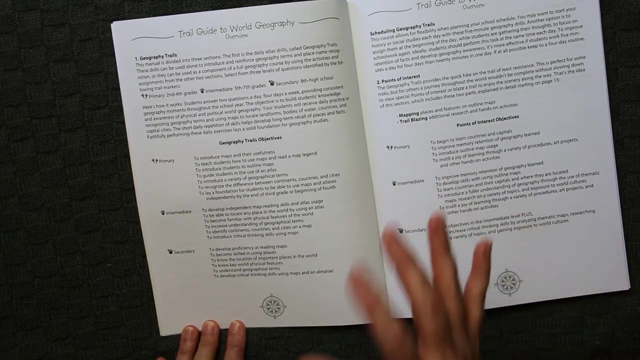 and make it a fully fledged, year-long, fully immersive geography program. So the overview pages explain the program And show how to break down the lessons for each child depending on where they sit within their grade level or age appropriate levels. So this is how you can easily make this program work. 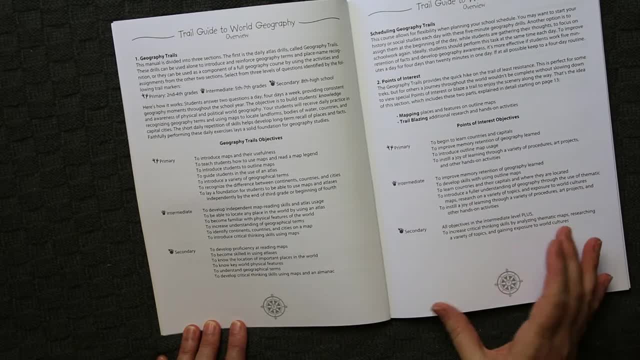 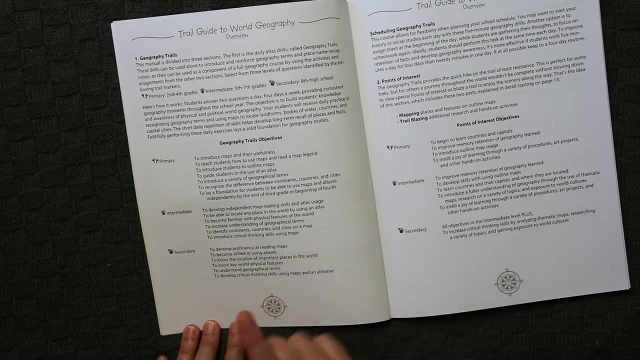 for a family and all work on it together, As each child will be given options that generally best suit their age and ability. So here's how that works. What you need to take note of are these animal tracks that you can see here down the sides. So have a look. here we've got which look. 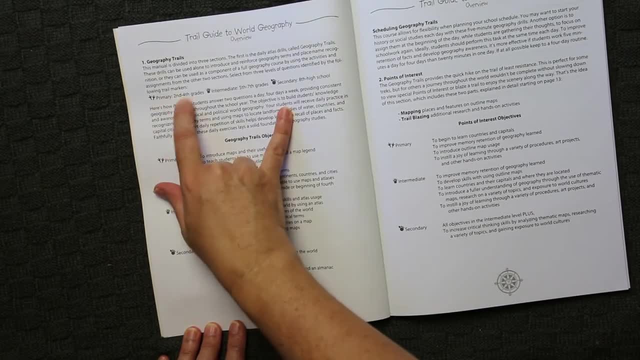 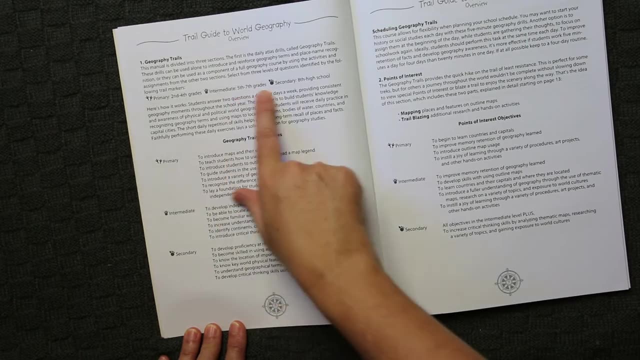 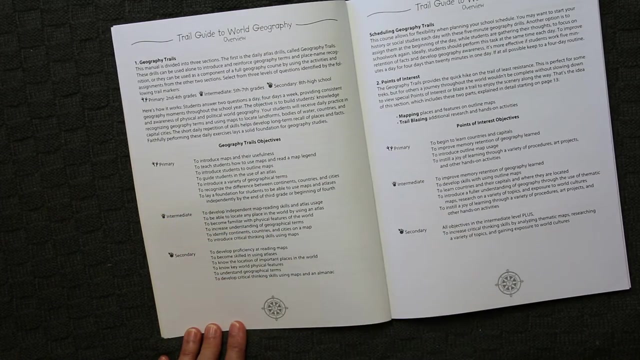 like some little bird tracks. These are level is aimed at the primary grades, roughly second to fourth grade children. Then you've got the intermediate fifth to seventh grades and secondary eight through to high school. So we need to take note of the little animal tracks. 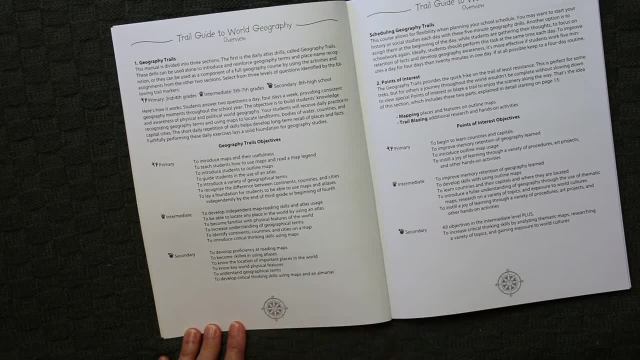 that pop up through the program. So if you're working mostly from the primary section, then you really only need to be concerned with what's here near the bird tracks And it gives you the overview or the objectives of the program for each grade. The geography trails are: 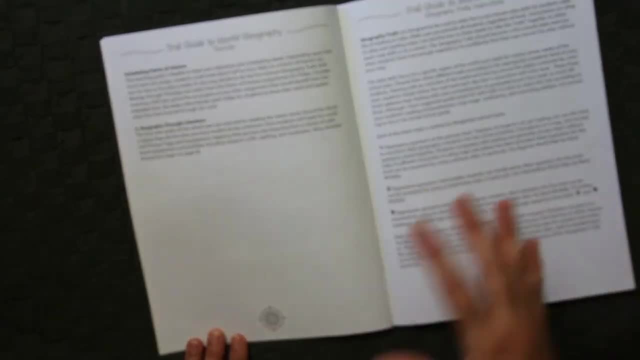 the mapping component of the program. So you'll need an atlas, and possibly one for each child, depending on how you want to work with this guy After the initial period of settling the child into using an atlas, where you may need to spend time with them every day for the first week or two. 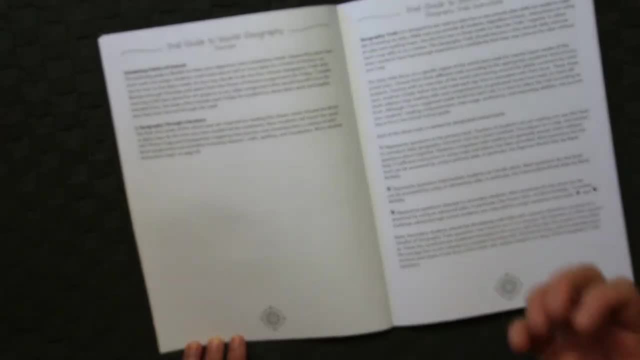 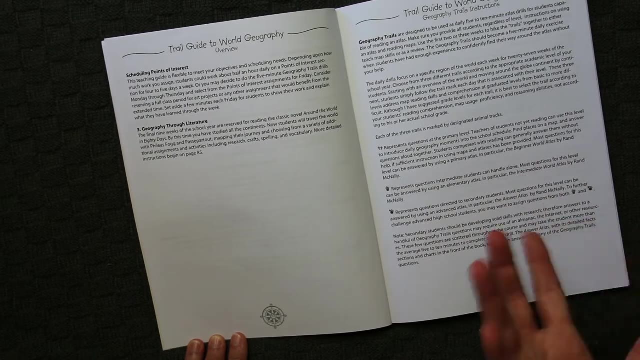 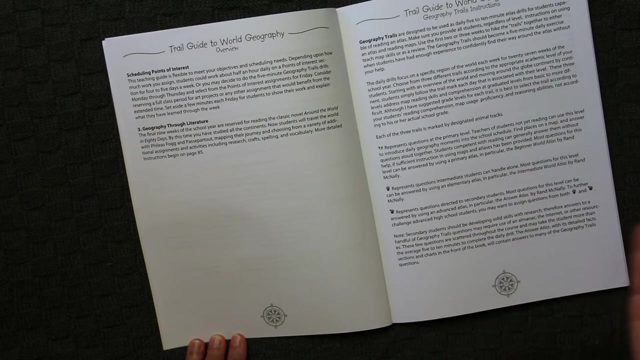 so that they understand how an atlas works and how to use the particular atlas that you've purchased. This part of the program genuinely becomes quick, five minute daily exercises. The guide does give suggestions for particular atlas to use, but it's not imperative that you have that actual atlas as. 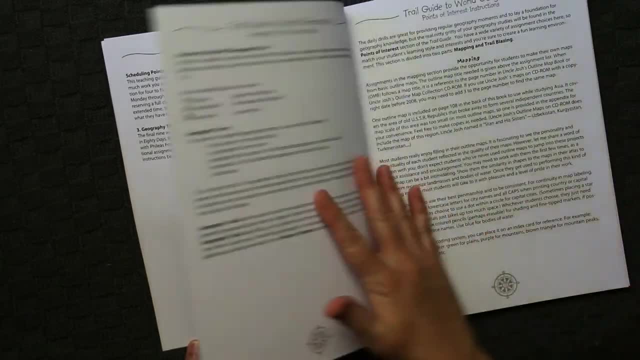 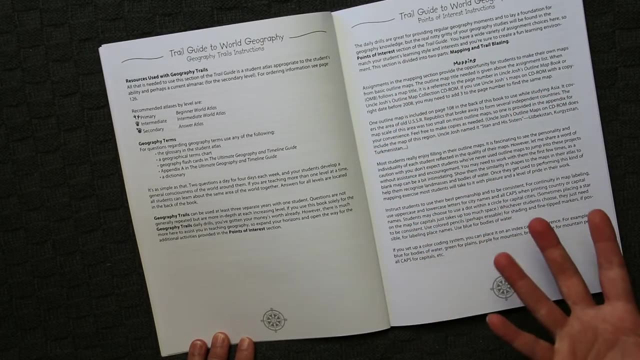 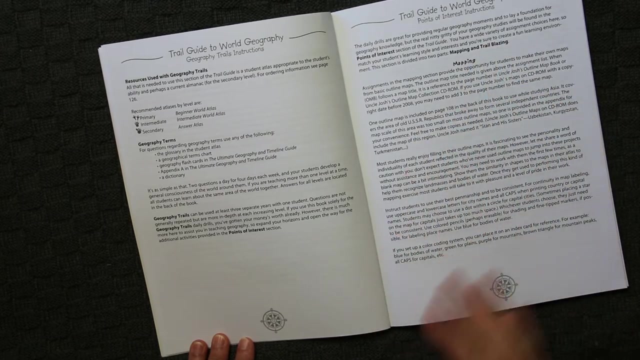 you can see here. And then we're moving on to the points of interest section and in the guide, this will offer a variety of assignment choices for the student, and this section is broken into mapping and trailblazing. Okay, so there are recommendations of other books that include mapping activities, but I don't feel. 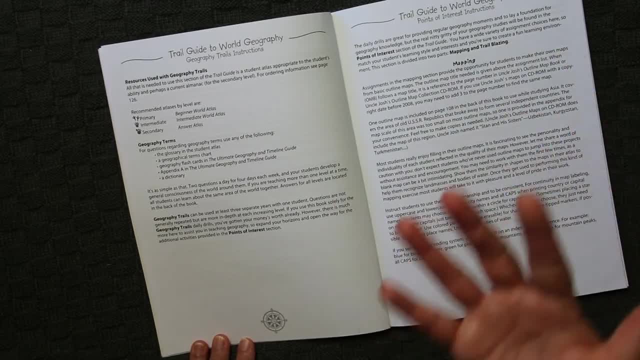 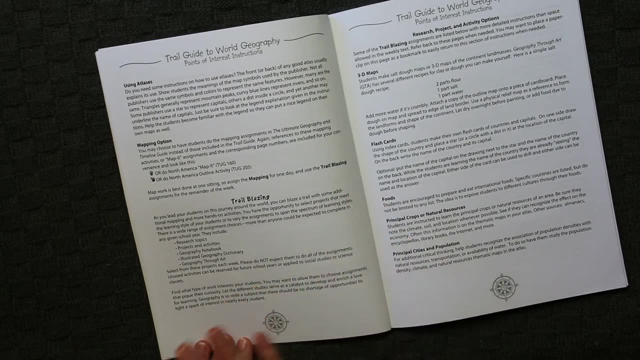 that they're imperative to the program. It's going to be a personal preference for you. After a mapping exercise, you may choose one of the trailblazing activities, and these can be things like research projects, 3D map making, looking more closely at natural resources, or cities, landmarks. 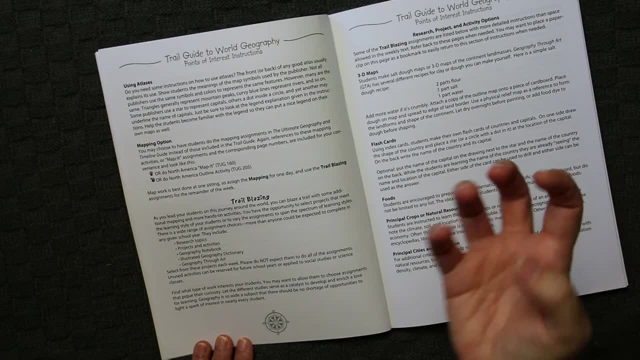 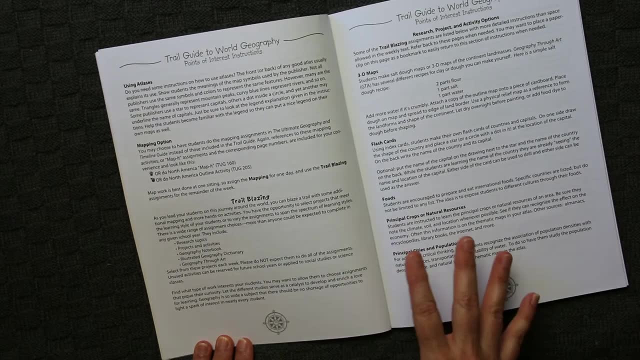 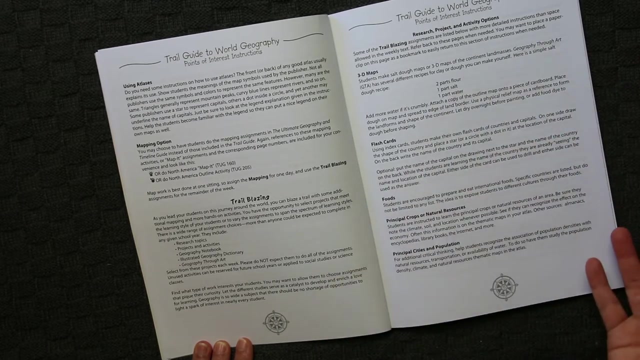 animals. Whatever the child is interested in when you're in that particular country is something that I would suggest You run with. There are also instructions included on making a geography notebook for each student, and they do offer an optional student notebook that can be purchased via their website. 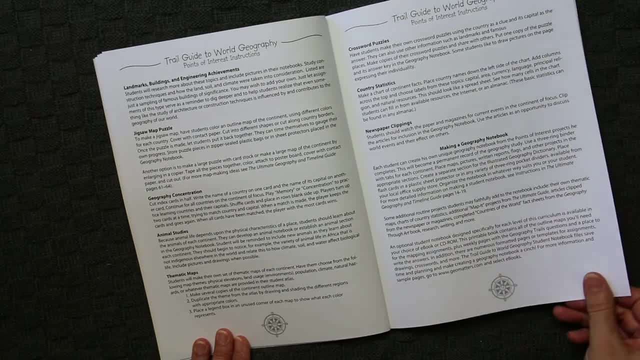 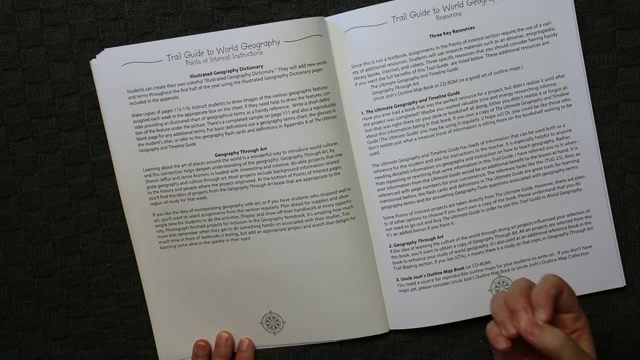 So, whilst not absolutely necessary, if you wanted the full benefits of the trail guide, then adding in these three key resources will, of course, round out the program. So, like I mentioned, there are things like an atlas, an encyclopedia, access to the internet. They are all going to be. 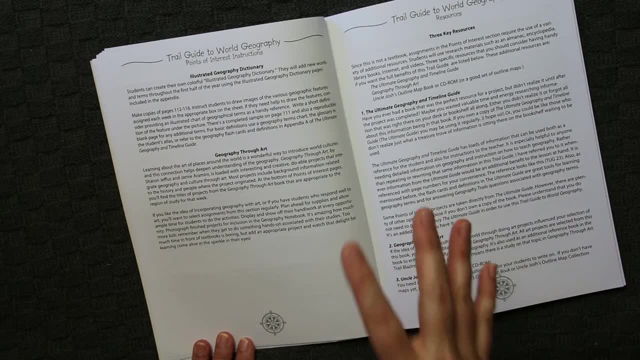 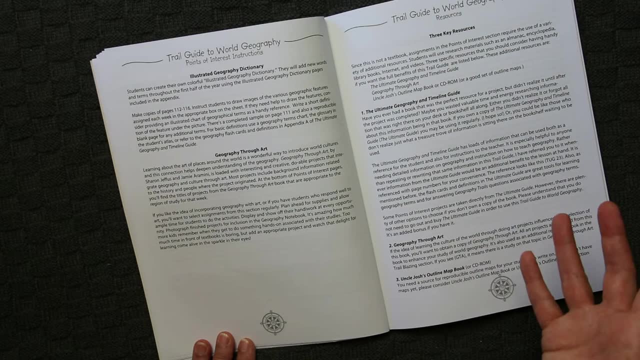 included in the trail guide And you will manage the whole thing as a whole. So let's get into these. going to go a long way in helping to conduct further research when the guide suggests, But the other key resources that the guide does recommend to use if you wanted to make this. 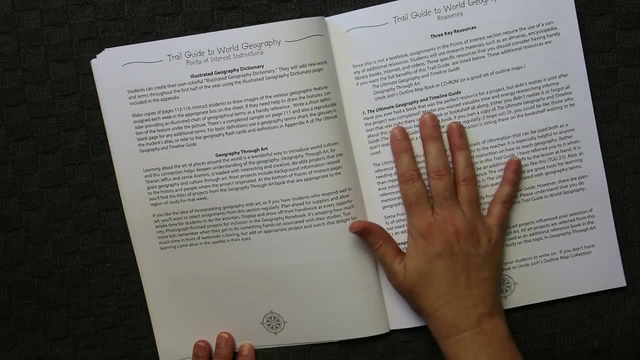 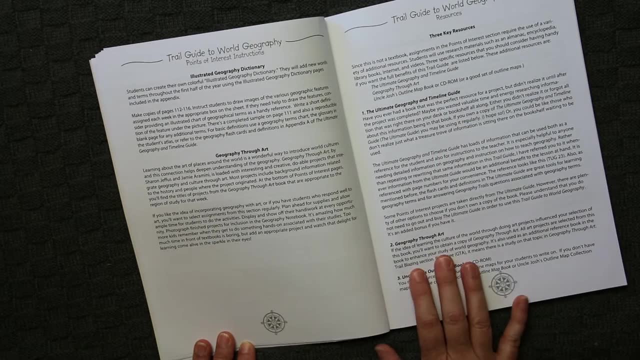 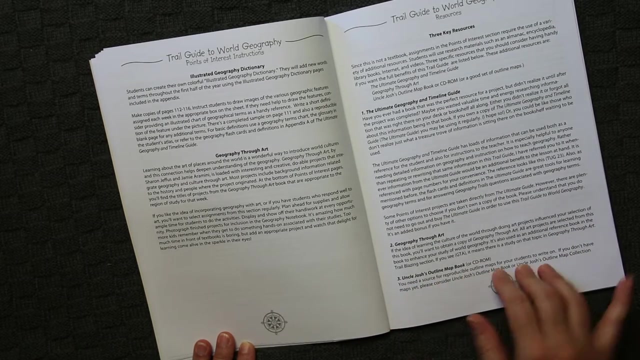 an all-encompassing program is the Ultimate Geography Timeline and Guide. This provides more detailed information on geography. Then we have Geography Through Art, which is a book to guide through learning about various cultures through art projects, and Uncle Josh's Outline Mapbook, which gives you access to all manner of outline maps. So, moving our way through the guide, 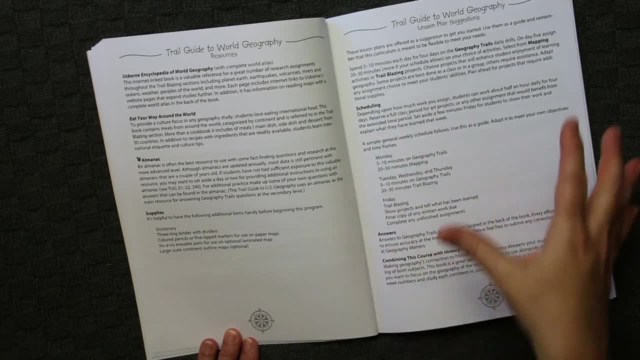 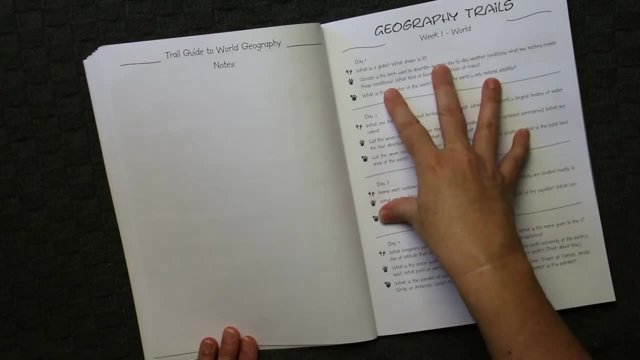 you will see that they offer suggestions around lesson planning and how you might like to schedule that in your week. Let's jump straight in to a lesson or two here. Okay, so we're going to start week one with the lessons straight into a geography trail. So straight away what I really 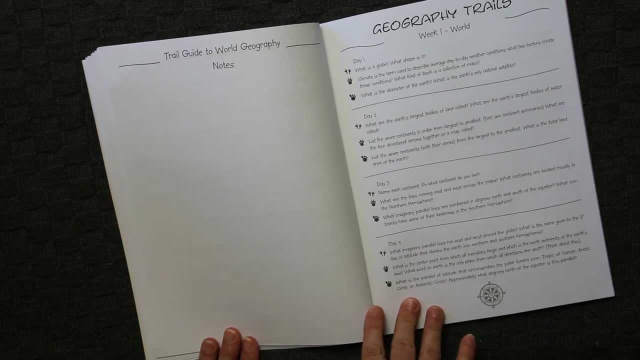 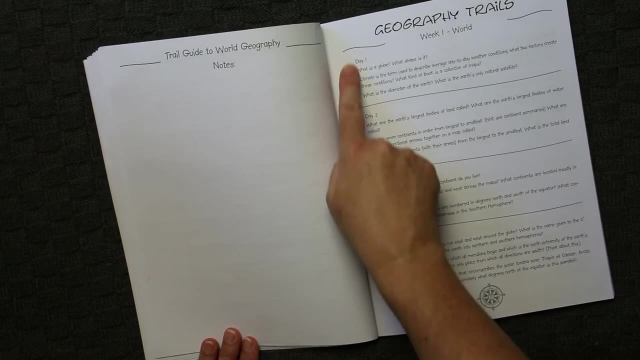 like about this guide is the ease of use. So if you're interested in learning about geography, which everything is broken down: A week is four days and then each day is broken into the recommended grade levels. So remember our little animal tracks that we're looking at here on the 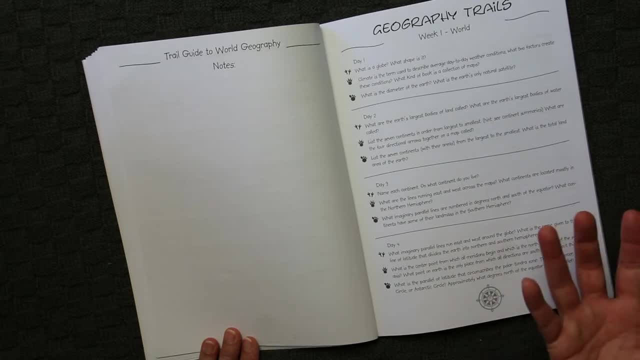 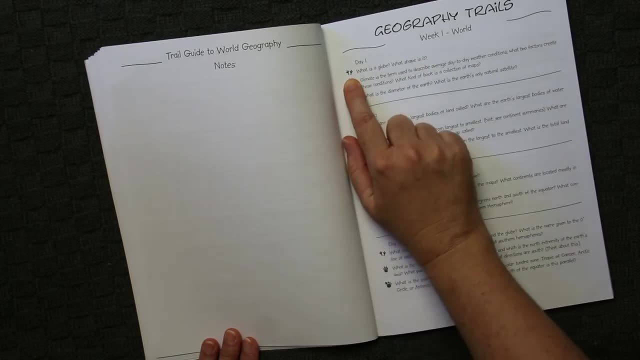 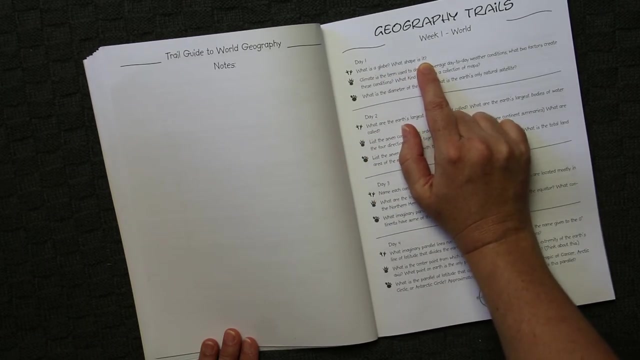 side. So, depending on what you've chosen, you just need to find that particular animal track, and that's what you're requested to do for the day. So, day one. for our younger students, it's simply a matter of what is a globe, what shape is it? So, of course, the parent can just 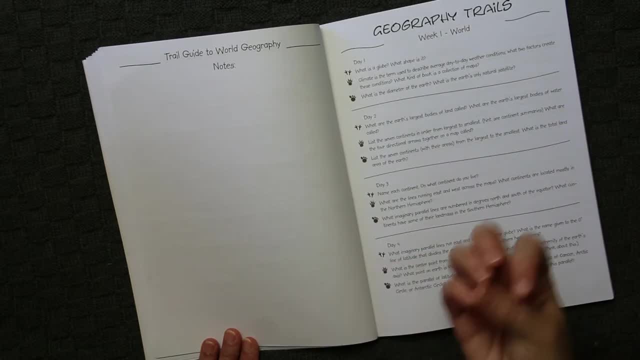 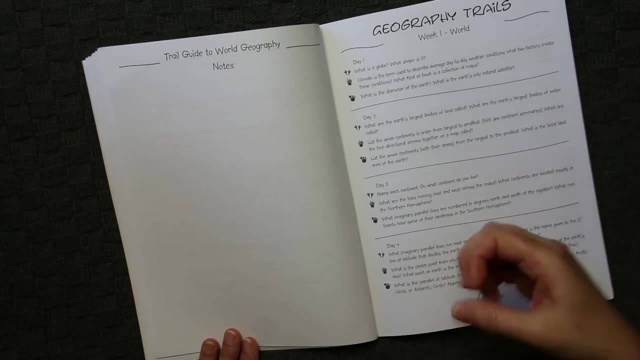 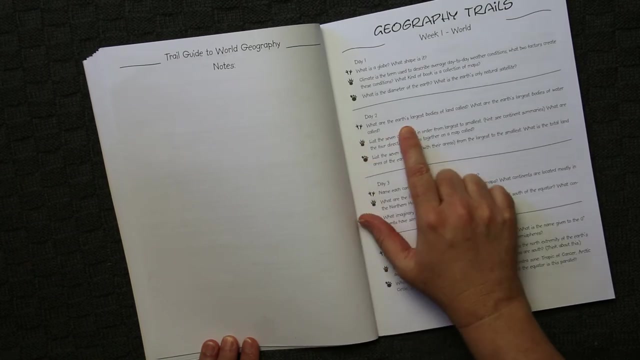 direct the child with that. You may choose to do this simply as discussion only, or you might want to add something to a geography notebook- you know a picture of a globe, or a child might like to draw a globe as best they can. Day two for the child, of the same level: what are the earth's largest? 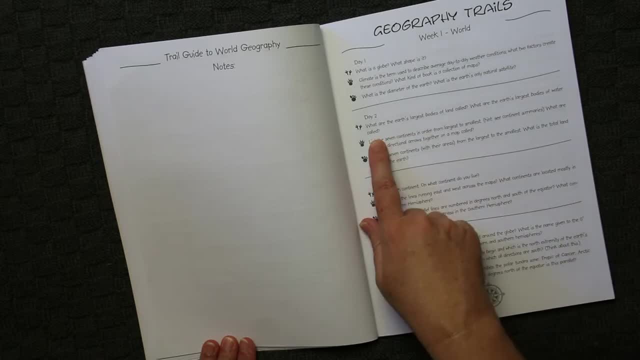 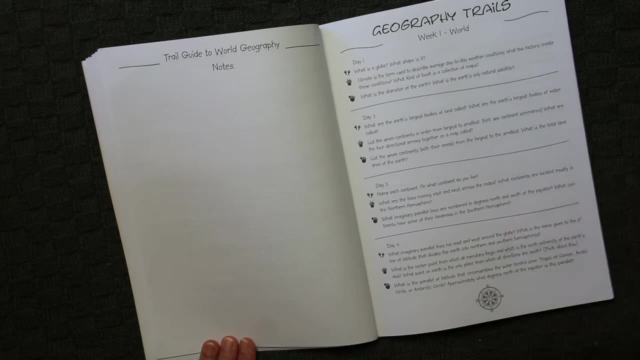 bodies of land called. What are the earth's largest bodies of water called? So here we may need to get out a book or an atlas and look for that information for the child, And again, up to you how you tackle that. So if you're interested in learning about geography, you might want to. 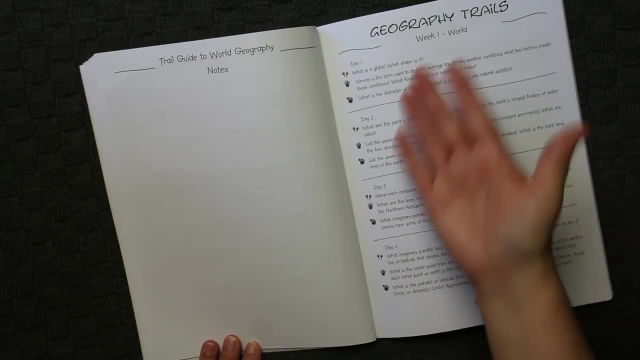 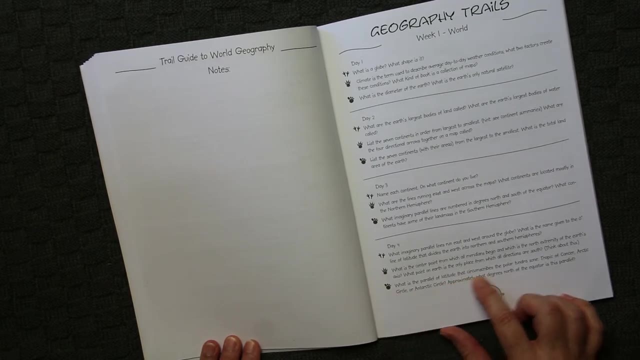 tackle that and whether you want to add that to a geography notebook. So let's pull out one of the higher grades. So let's look at high school on day four. What is the parallel of latitude that circumscribes the polar tundra zone? Tropic of cancer, arctic circle or antarctic circle? 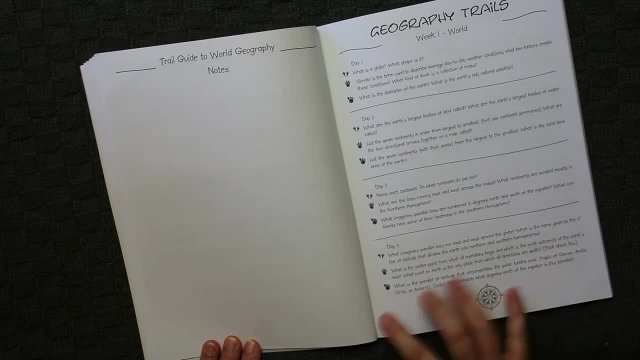 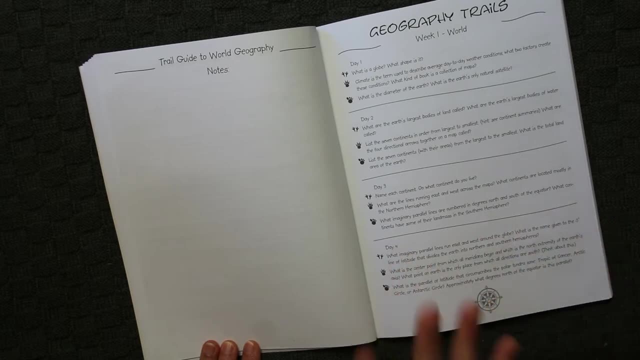 Approximately what degrees north of the equator is this parallel? So, as you can see, it's definitely got the children diving deep into getting to know their atlas really, really well. Then, over the page, you will have what they call, of course, their points of interest. 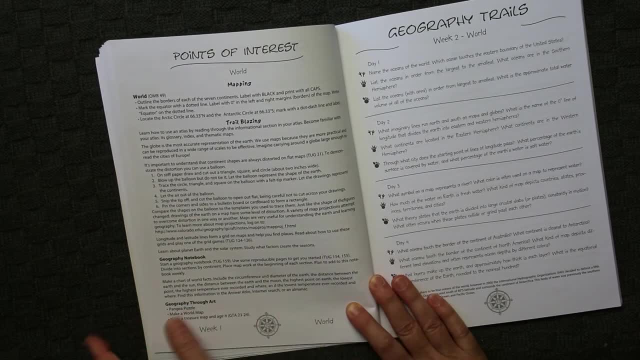 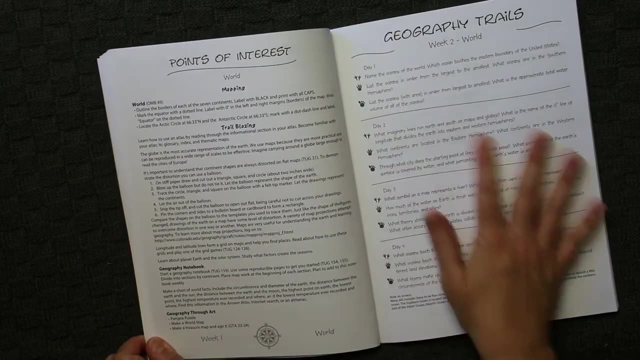 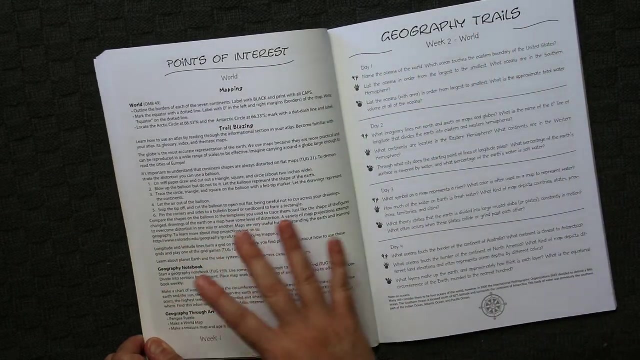 And this will list you a whole bunch of ideas that you could do. This is the great thing about this particular guide: The actual lessons are really short and to the point, but you were then provided with all of the ideas where you could extend things whenever you wanted. So on days that. 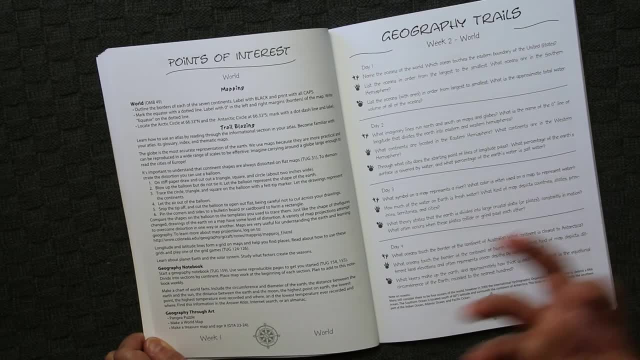 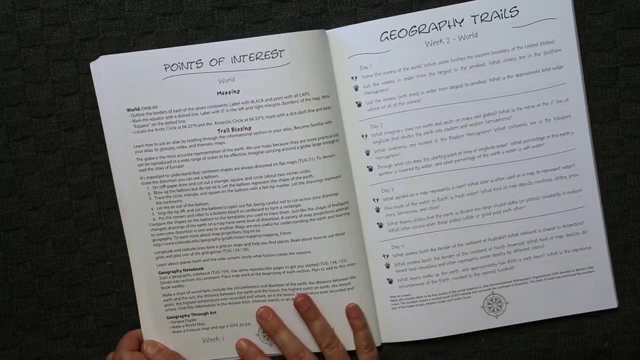 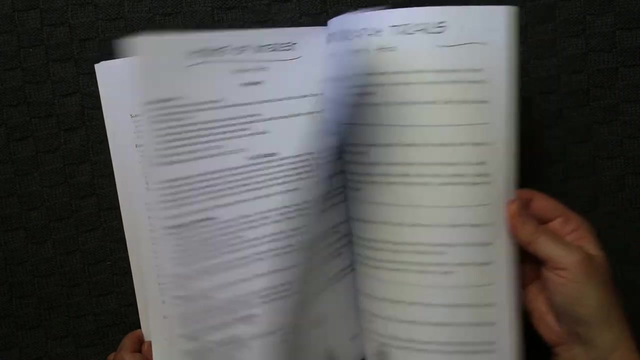 you know are short on time, or you know mood is low or any of those things. doing this is sufficient. But if you want to spend more time, you've also got a whole gamut of ideas to extend on. So if we flip further into the book and take a look at how things progress, 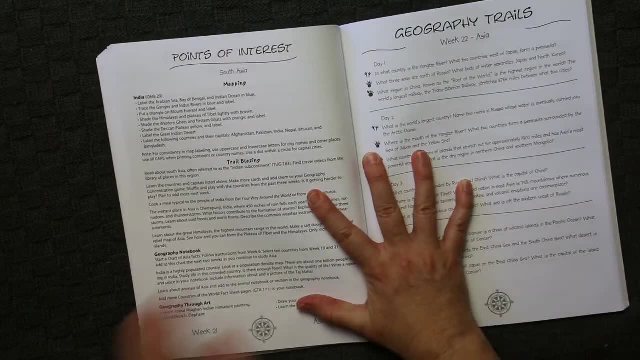 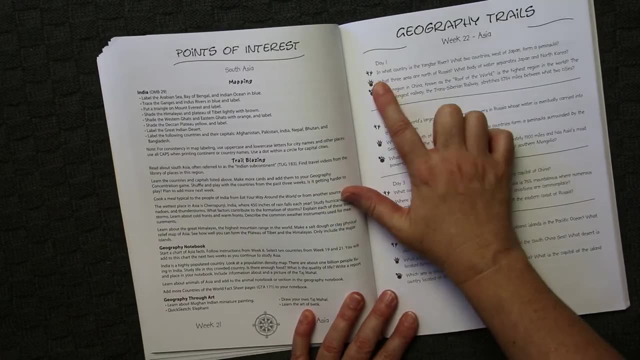 So let's go up to. let's have a look here. We're at week 22 and we're in Asia. So week 22,, day one, we're still looking at our younger children. In what country is the Yangtze River? What two countries west of Japan form a peninsula? 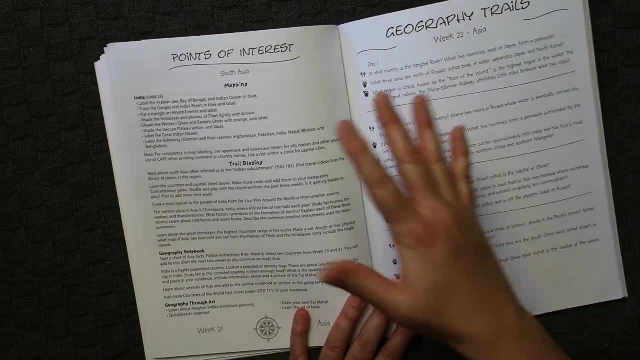 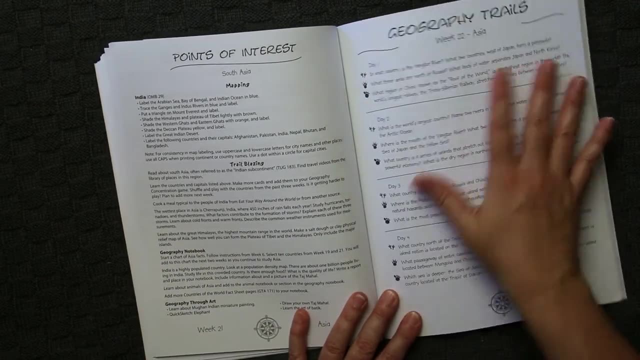 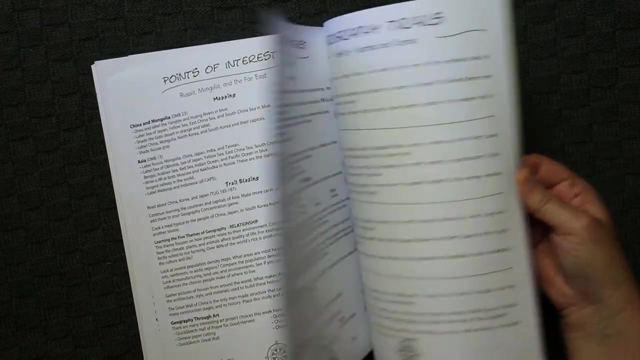 Now we are at week 22 here, so you would expect that the child has built up enough skills to be able to use their atlas to find this information And of course, if they can't, then you or an older child can sit and work through that with them. Then if we flip through to week 28,. 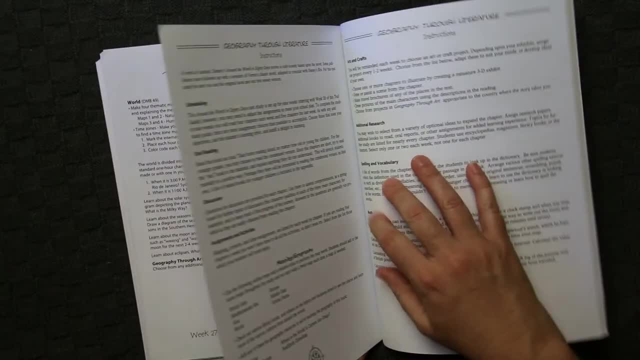 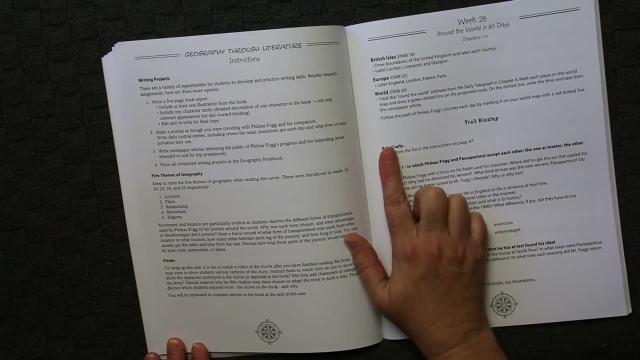 it tells us about where we are and how we are living out these conditions. So we have week 28,, times four, and憲 will see that we bring in a literature study gives a little few instructional pages prior to that, but we're looking at around the world in 80 days and then